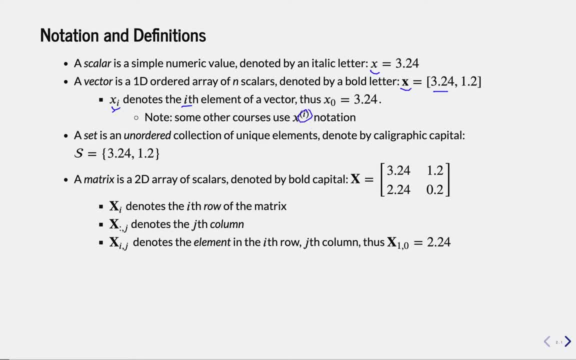 notation like this, but we'll just stick to the sub notation. Whenever you see a curly letter s or a set of numbers with curly braces- that is a set means that these numbers are unique and ordered. A bold capital letter x, that means it's a matrix, which is a two-dimensional array. 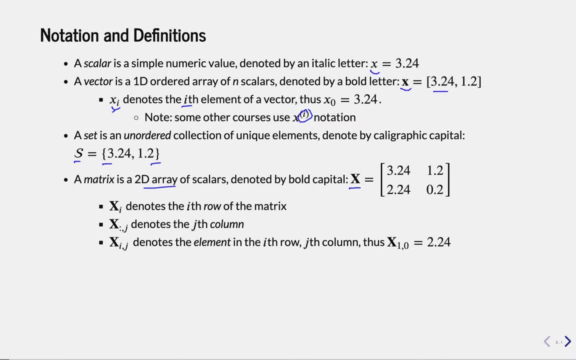 of scalars: x sub i means the ith row of the matrix, x, colon j denotes the jth column of the matrix, And x sub ij denotes the element in the i-th row, in the j-th column. So whenever we see x 1- 0, it means row number 1, that's this one and column 0. 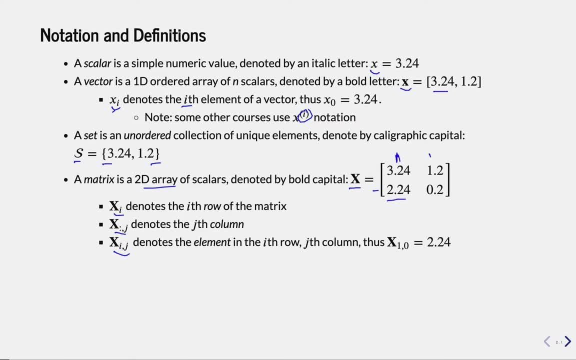 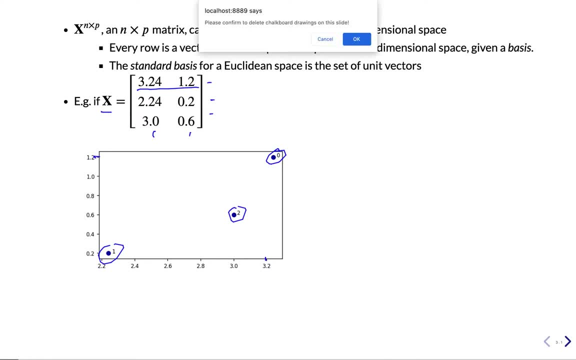 it's this one, So we're looking at this value here Now. matrices typically have a geometric interpretation. Whenever we have a matrix N times P- that means it has N rows and P columns- then this matrix represents N points in a p-dimensional space, according to some basis, but typically we talk about 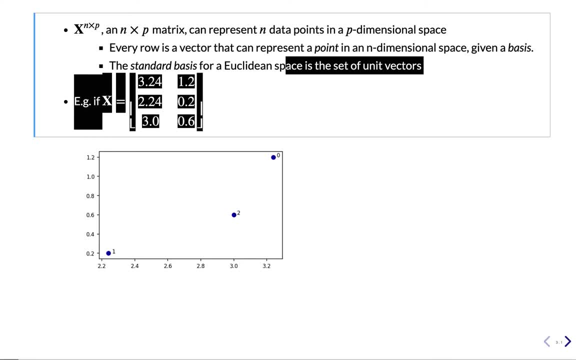 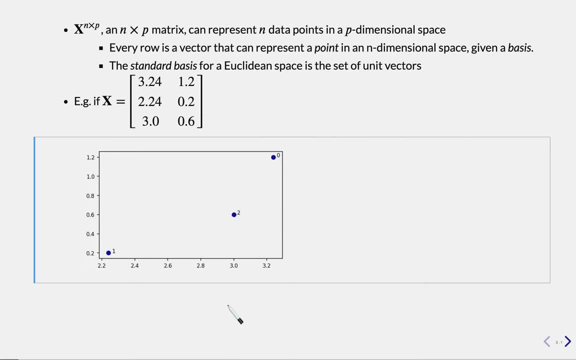 euclidean space, For instance this x here. so the first element here is the euclidean space, For instance this x here. so the first element here is the euclidean space, For instance this x here. so the first element here is the. 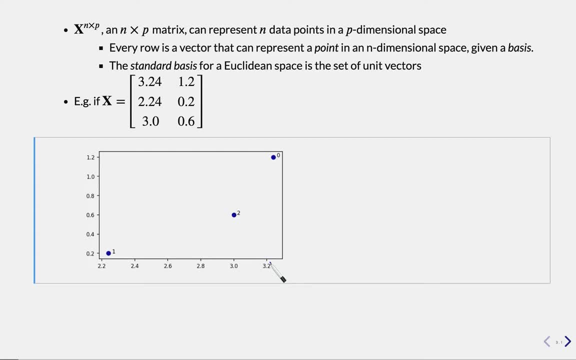 3,, 2,, 4, and then 1.2,. so that's this one in here and that's this point here. The second one- 2,, 2,, 4, and 0.2- is this one here. 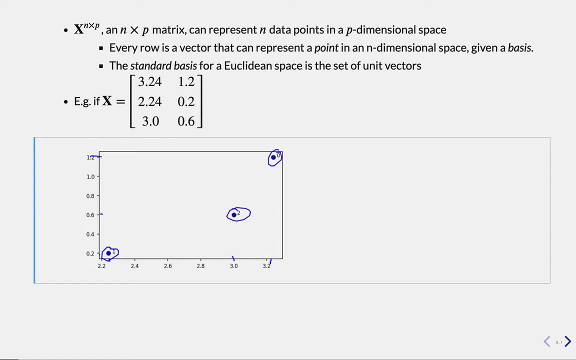 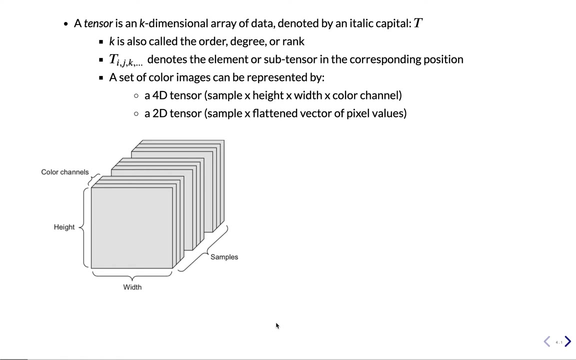 and the third point 3, 0.6. is this one right? So this represents basically a data set consisting of three points in a two-dimensional space. A tensor is a k-dimensional array of data, So one dimension is a vector. 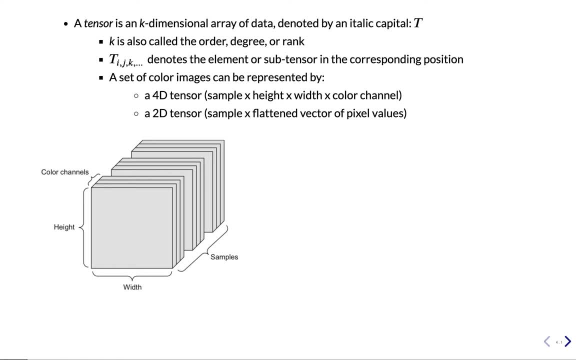 two-dimensional is a matrix, but more generally a k-dimensional array is called a tensor, which is denoted by an italic capital: T. K is also called the order or degree or the rank, and whenever we see italic T, I-G-K means it's the element of a tensor. 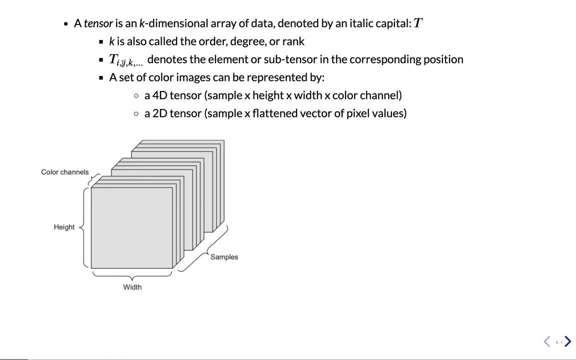 in the A position in the first dimension, the J position in the second dimension, the K position in the third dimension, and so on. One typical example is a set of colored images, So whenever we have an image, this can be represented by a height and a width. 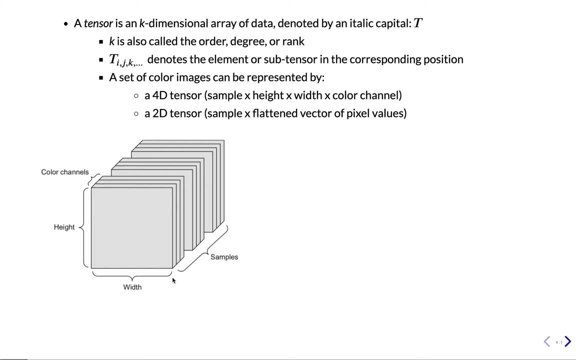 So this image has a height and a width, so every value here is a pixel. That image also has color channels- red, green, blue- and there are multiple images in the data set. This is, then the fourth dimension. right, We could also like. 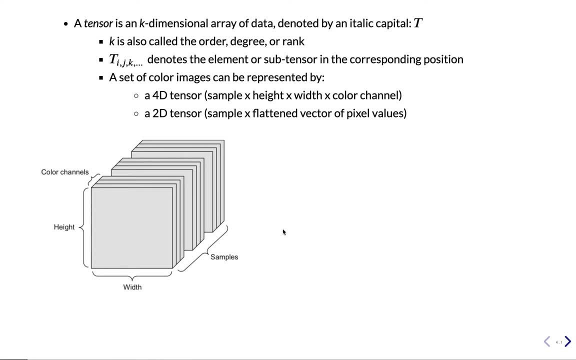 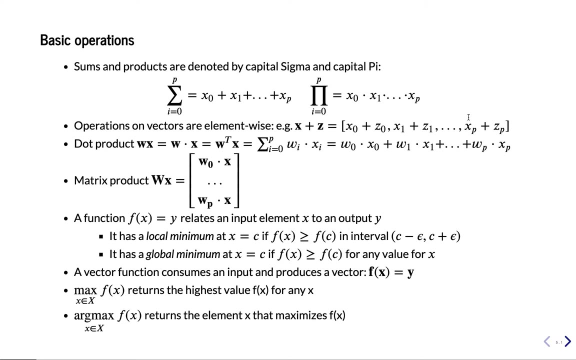 flatten this two-dimensional array as one vector, but then of course we lose some of these relationships between the values, So it's typically then represented as a four-dimensional tensor. Some basic operations which you will often see. So first, whenever we see a capital Sigma, 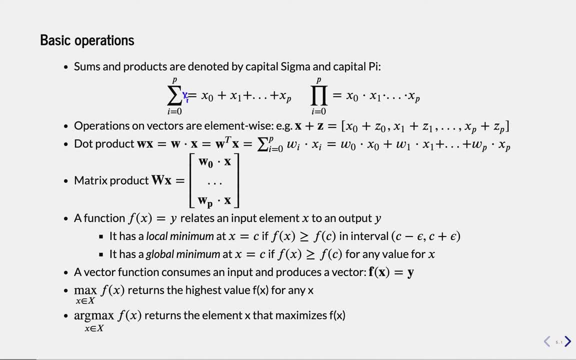 that means the sum. So capital Sigma of X-I means we take the sum of all the elements in that vector X. The capital P means we take the product of all the elements of vector X. If you take the sum of two vectors, that is a new vector in which every value 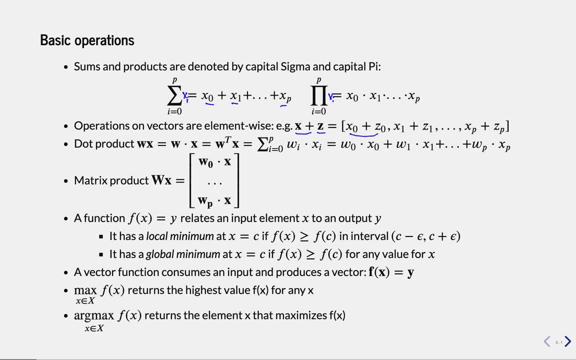 is a sum of the values of the corresponding vectors. A dot product denoted by two bold values, Letters WX for instance, it's a dot product. You can also see this in the dot notation or the matrix notation, but we'll typically stick to the simple notation like this: 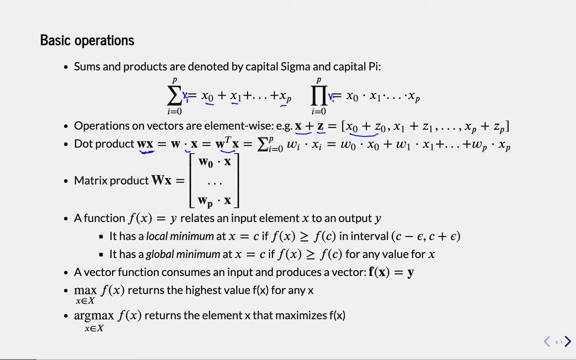 This is a number. It's actually the element-wise product, like W0 times X0, W1 times X1, and then we sum up all these values and that is a dot product. This has a very well-known geometric interpretation. 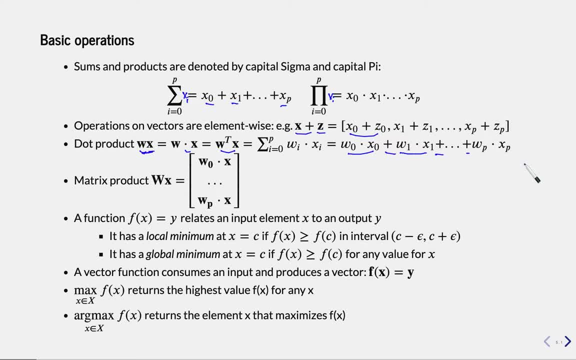 for instance, if you have two points- W and X- according to some basis, then the dot product is basically the projection of this W on X, like this, which means that this somehow tells us that the two points are close together. So if two points are close together, 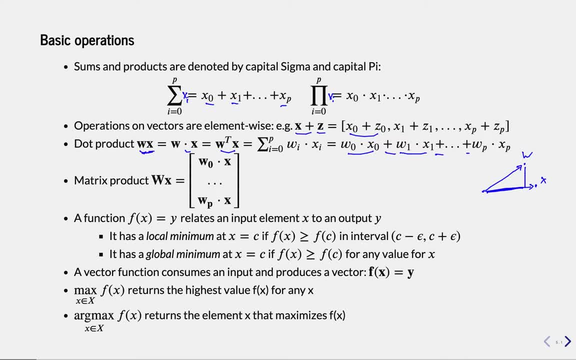 the dot product will be large. If two points are far apart, the dot product will be large. If two points are far apart, then the dot product will be very small, And this will be often used in this course, so remember this. 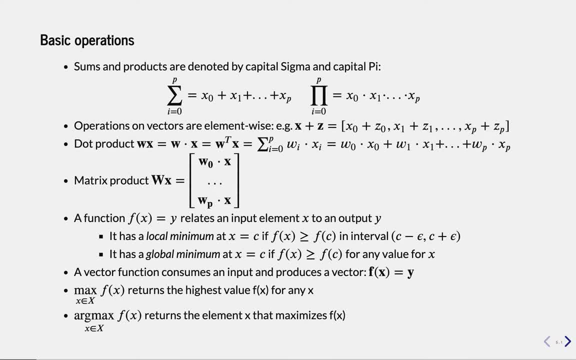 Whenever we have a product of a matrix and a vector, the result is a new matrix in which we take the dot product of every row in the matrix with that vector X, so it has input X and Y. If and when we have function's in 완� després de ces exposed четters. 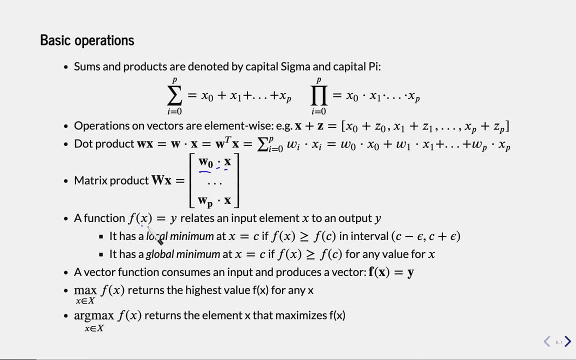 every node has the output Y workingئ. Whenever the function has a minimum, that's any point c where in some area around c every other point is larger, that's a local minimum. Whenever there's no other point lower in the whole domain function. 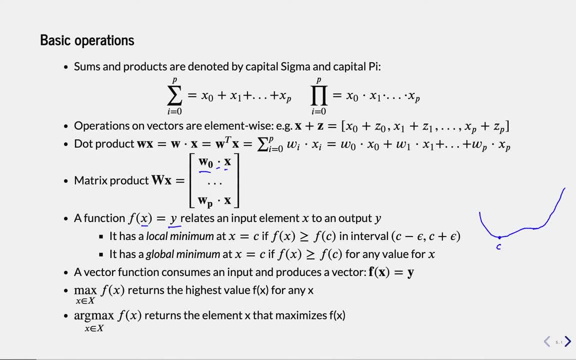 or in the full domain of a box. then every other point of the function is larger and larger. then this is called a global minimum. All right, so you can imagine some point here. this could be a local minimum. this is the global minimum. 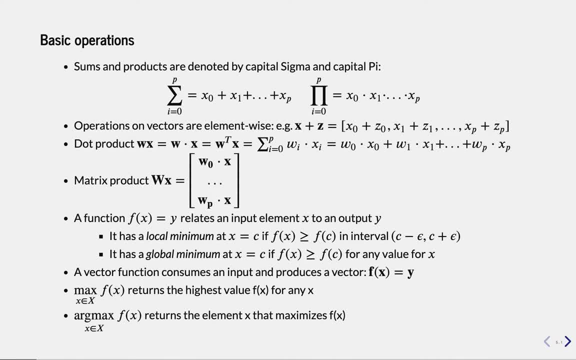 Some functions output a vector. so whenever you see a fat function f, it's a vector function which has input a vector and also output a vector. Then if we have a function x, y which has a maximum, we notate the maximum like this: 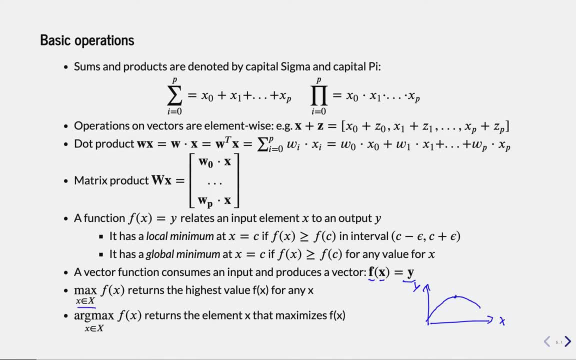 so this is the highest value, the value of x. sorry, it is the highest point of this function f, that's max, Arc. max is the value of x, which corresponds to this point here, which corresponds to the highest value of function f. 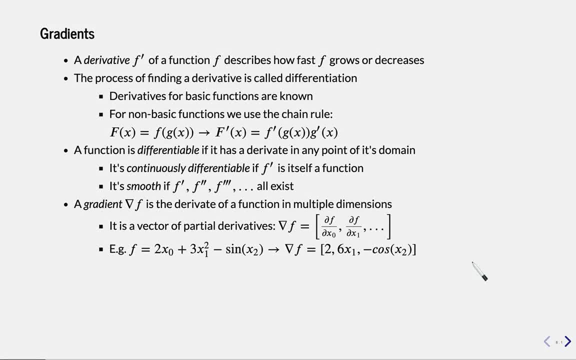 Now, a very important concept in this course are gradients. To explain gradients, let's first consider a function, f and function of x, And say that this function is x squared looks like this, Then then the derivative of this function: 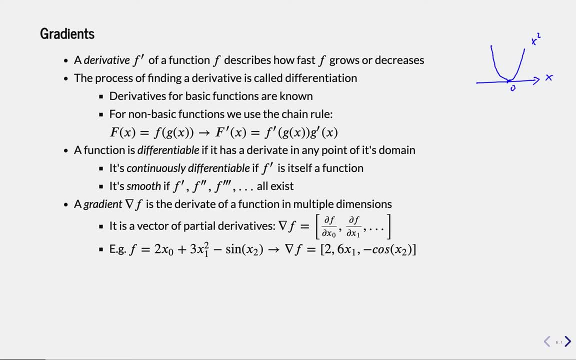 this function tells us, at each point x where this function is going down and by how much. Typically, we can compute this derivative using some basic rules. The derivatives of most basic functions are known, So we know. the derivative of x squared with respect to x is two x. 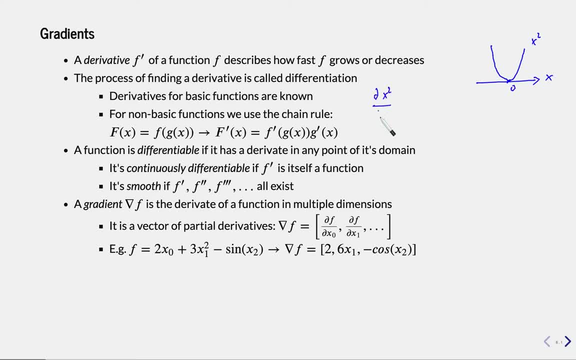 So the derivative of x squared with respect to x is two x. So this function basically tells us how this function is evolving. So x two looks like this. So this tells us basically the slope of this function. So if you take a function point here: 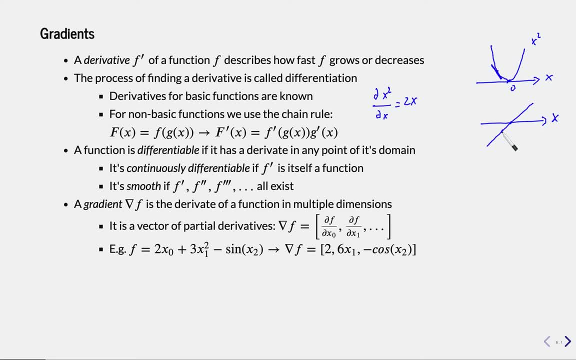 the slope tells us that it's going down and the gradient tells us, yes, this is indeed going down, because this is a negative Like this could be like minus two, for instance. here This is going down At this point, here it's going down a lot right. 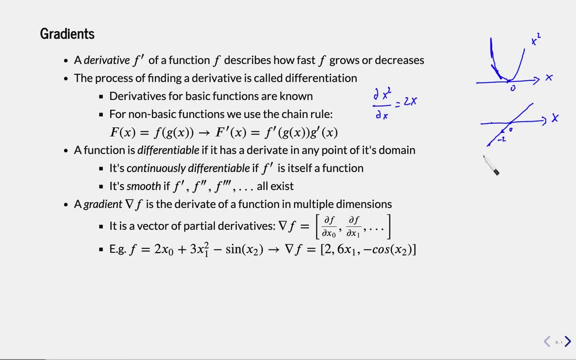 So then you can say: okay, here this could be like minus 10,, okay In the other direction. so here it's zero, The gradient is zero, The function is stationary in that point, And on the other side, here the gradient goes up. 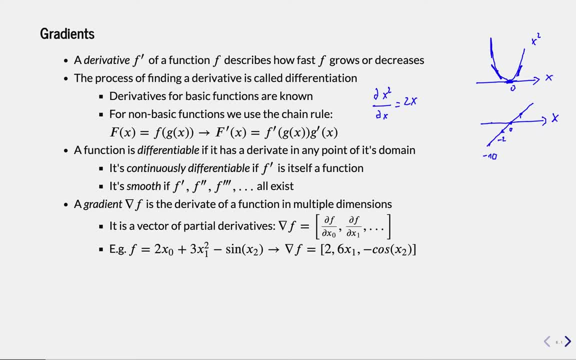 So the gradient is positive. Okay, Function is. so. whenever we have a more complex function, for instance a function where we have an outer function and an inner function, g, then the derivative of this function is derivative of the outer function times the derivative of the inner function. 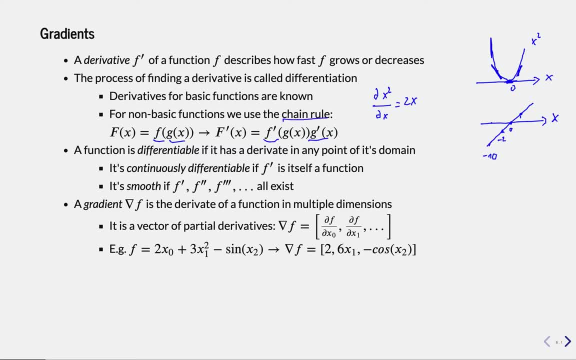 It's called a chain rule. It's very useful. Now you say the function is differentiable if it has a derivative in any point of its domain. So a function like this, at any point we can compute the gradient. So this is differentiable. 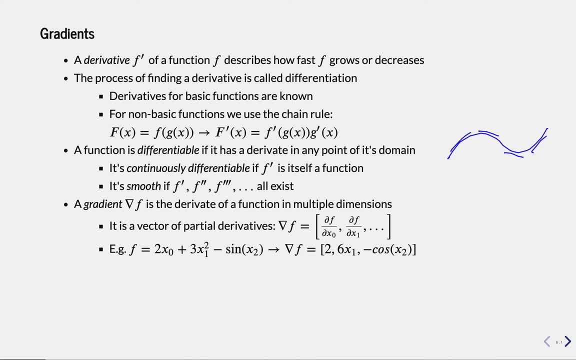 It's continuously differentiable. If the derivative itself is a function and if every derivative is also exists, then the function is smooth. Now, a gradient is basically the extension of this ID to multiple dimensions, right? So if you have, if x is a p-dimensional vector, 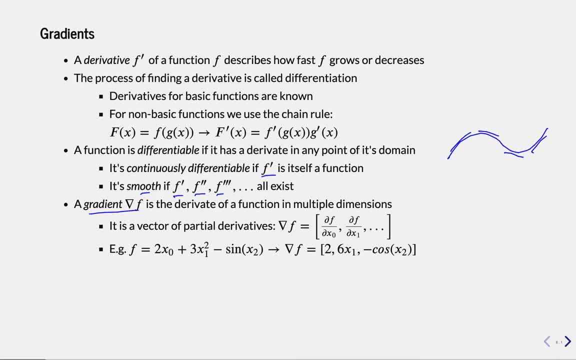 then the gradient is a p-dimensional vector And every element basically tells us what the, what the derivative is of the function according to a certain dimension. okay, So if you have, for instance, this function, f, then first of all we can compute derivative of f with respect to x zero. 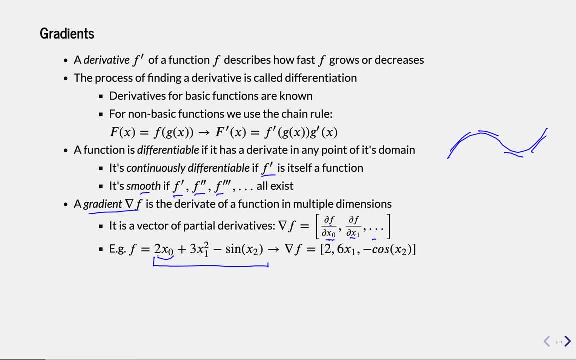 There's only one element which has a zero derivative, that is two. So the first element of the gradient is two Derivative of f. according to the second dimension, x, one. there's only one element. for this one, The derivative of this is three times two. 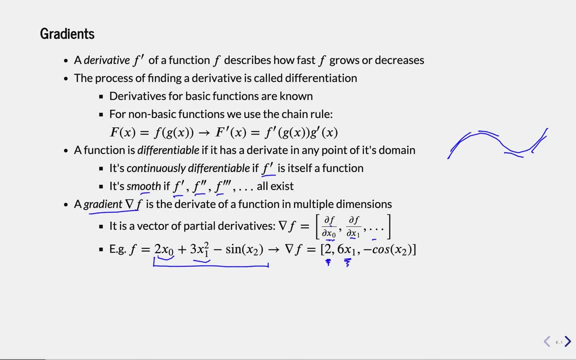 that's six times x one is this one? And finally, the derivative of f with respect to x two. this is the derivative of sine, this is the cosine, so this will become minus cosine x two. right, This tells us for every dimension. 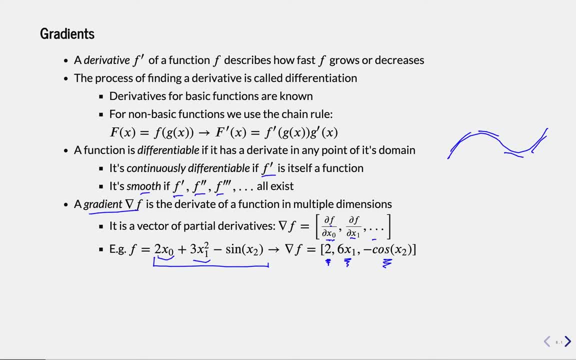 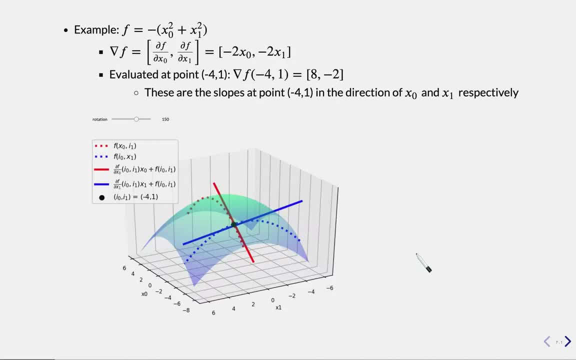 for every direction, basically how this function is changing. We can look at this also more geometrically. So say, for instance, we have this function, f, which is minus x zero squared x one squared. so we have x zero and x one. we have two dimensions. 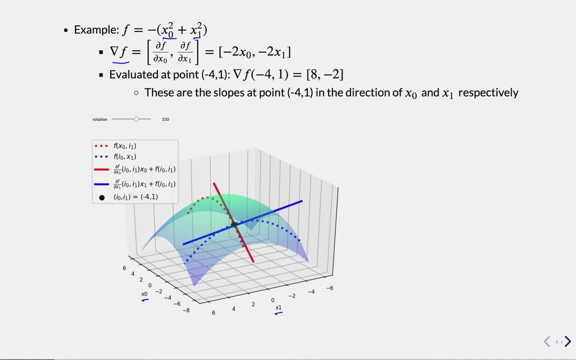 The gradient of this you can compute analytically. So the gradient of f with respect to x zero, that's minus two times x zero. with respect to x one, that's minus two times x one. like this right, This is the gradient. 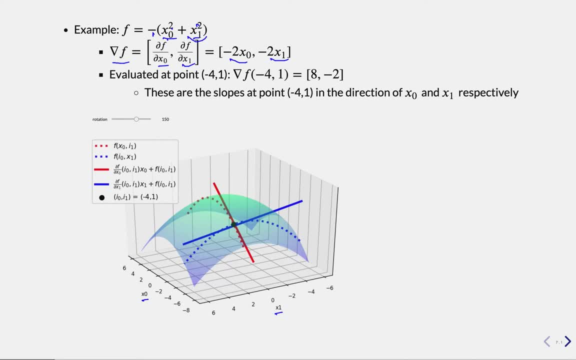 Now we can evaluate this gradient for every point in them. So say, we look at the value minus four, let's see it's here and one, that's this point. here the corresponding value of f. this is f minus four one. 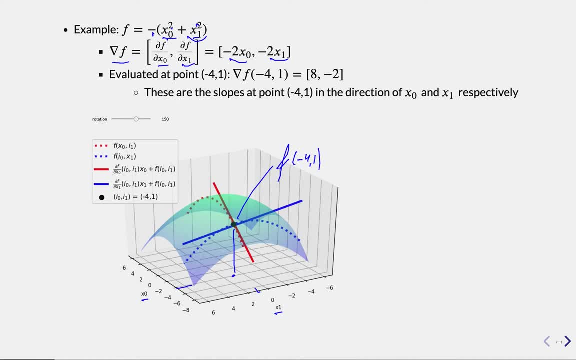 Now the gradient tells us how much the function is changing at this point with respect to x zero and x one. So it tells us with respect to x one: so if you do minus four times minus two, that's eight. So this tells us that as x zero goes up, 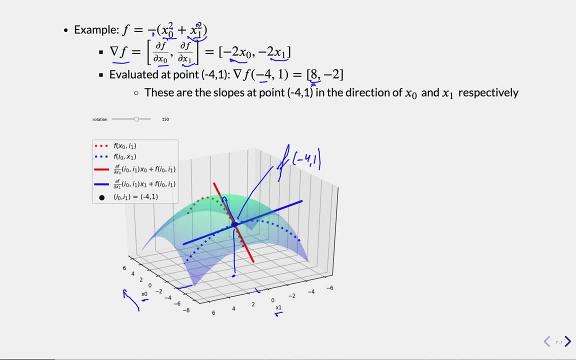 f goes up with a slope of eight right. So x zero goes up one unit. f goes up eight units In the direction of x two x one, and we do one times minus two, that's two, So the gradient there is minus two. 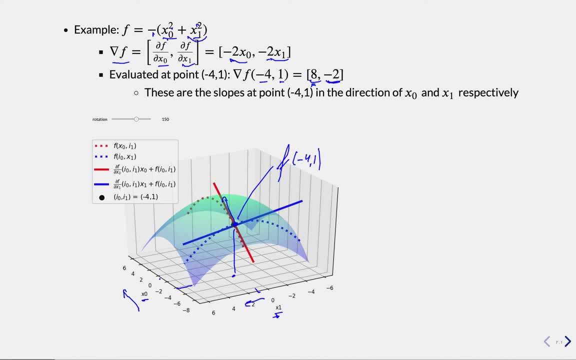 it tells us as x goes up, the function goes down with a slope of two. So this basically tells us in which direction the function is changing. sorry, by how much. the function is changing in every direction. If we rotate this figure we can get a better view of that. so say we want to look at the 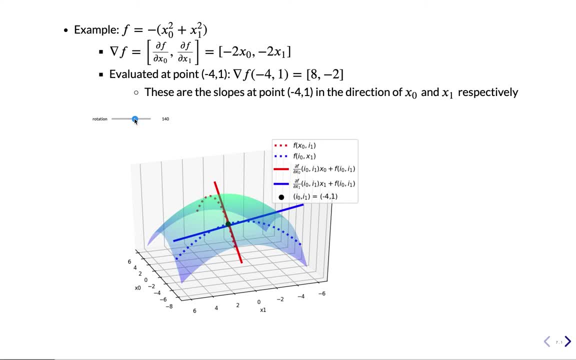 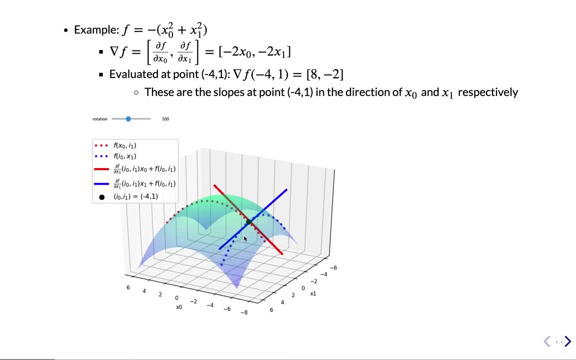 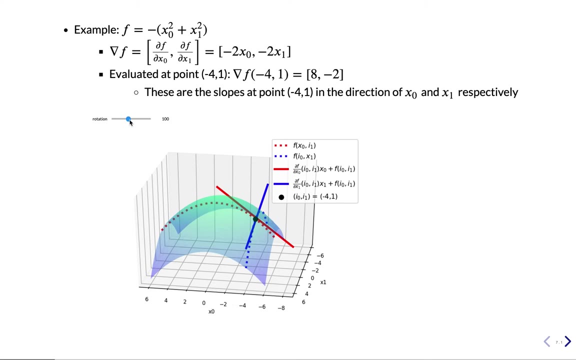 gradient for x0,. let's rotate this right, so now we can see that as x0 goes up, f goes up by 8 times that amount, right? so this is a very steep slope. and as x goes up, function. 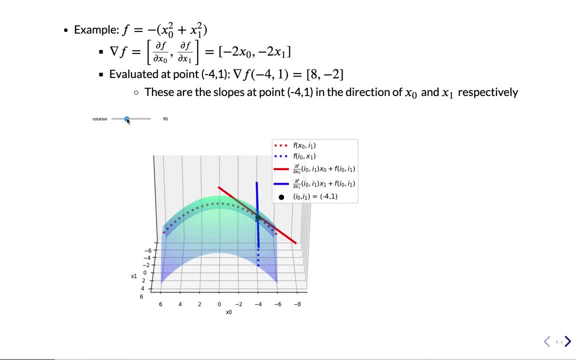 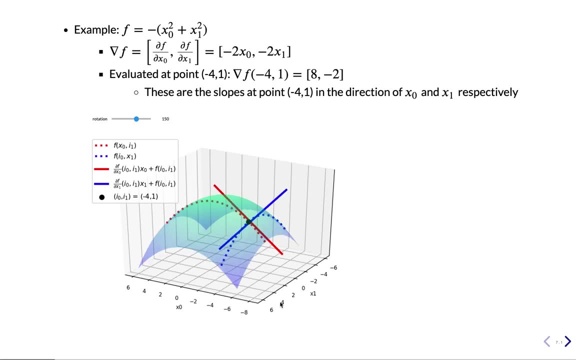 also goes up. That's the red line here With respect to x0.. Okay, With respect to x1, we said, as x1 goes up, this function here actually goes down. the slope is minus 2, so this tells us that the function is going down the direction. 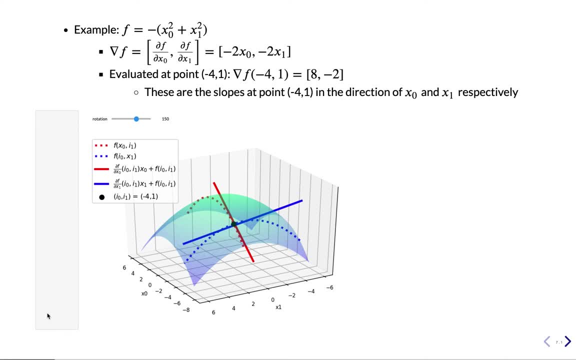 And this will be very useful whenever we want to find the minimum of a function, For instance in gradient descent. it will tell us that if we compute the gradient, we can basically tell: Well, we should go down by a lot in this direction and also by a little bit in this. 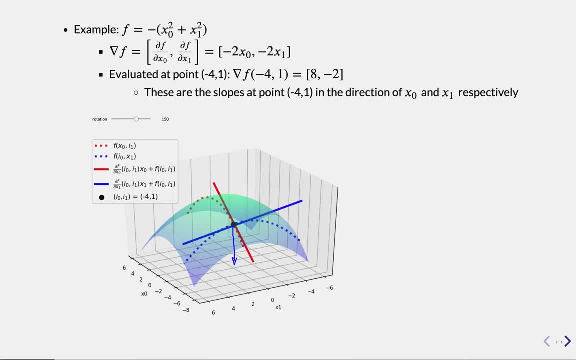 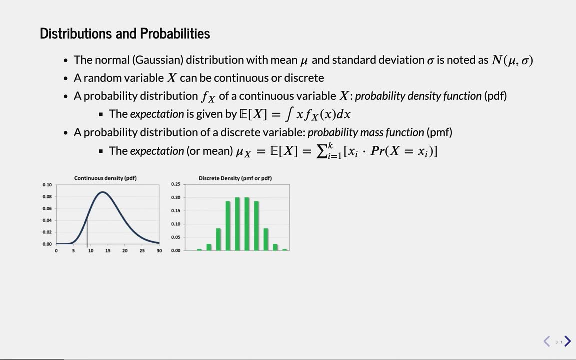 direction right. This is the steepest way down that surface. Finally, distributions and probabilities. so we'll often encounter the novel distribution or the Gaussian distribution. so obviously you know what that looks like. it's a bell shape, Okay.